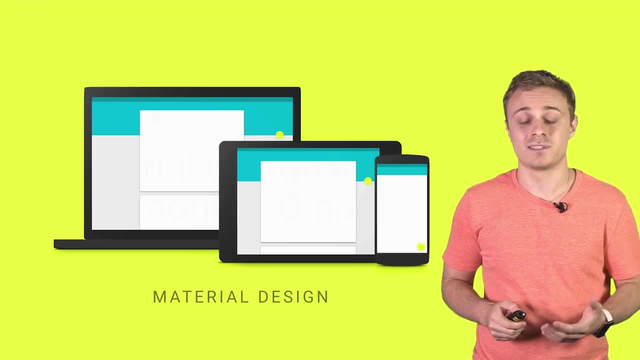 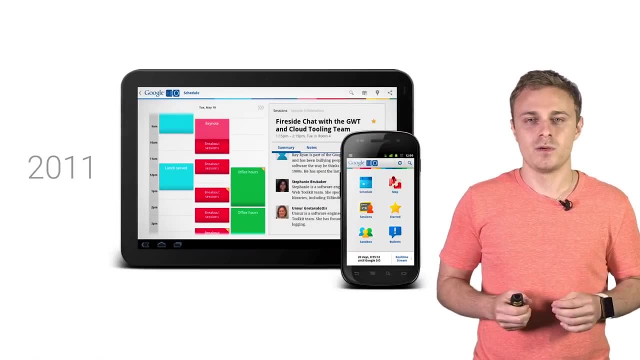 and motion design decisions across mobile desktop wearables and beyond. Now, every year at Google IO, our team spends several whole months working on the conference app. We do this for two reasons. First, it's obviously a great companion for the developers. 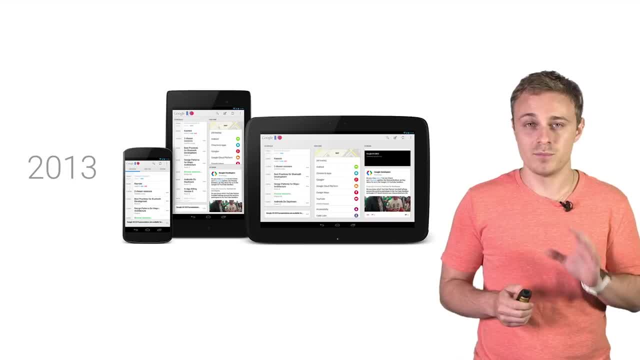 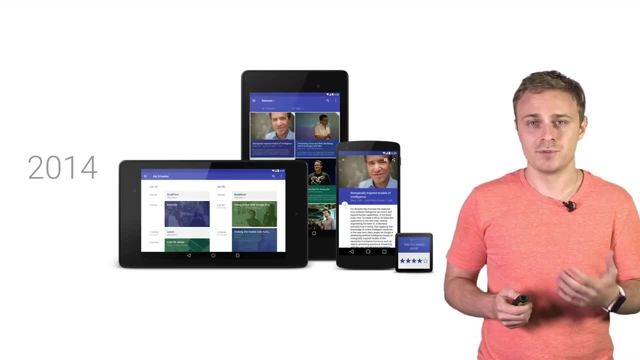 attending the event and those tuning in at home. Second, and arguably more importantly, it serves as a reference app for Android design and development best practices. Now this year's app uses Material Design and features of the L Developer Preview to present content and use it to develop a visual design approach. 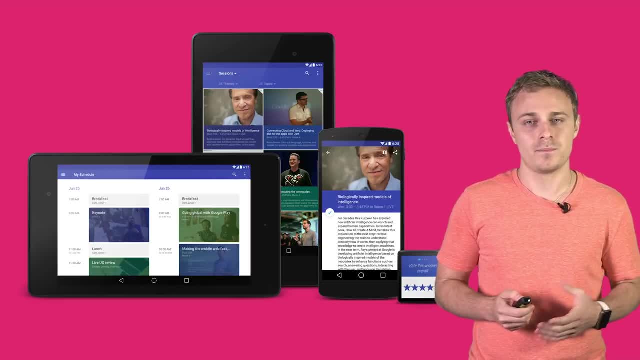 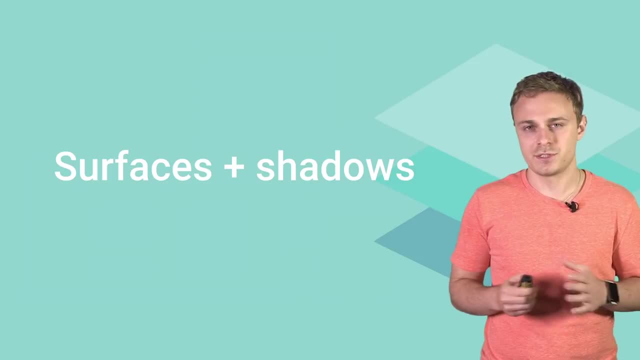 Let's take a look at some of the decisions and outcomes that informed the app's design. In Material Design, surfaces and shadows play an important role in conveying the structure of your app. The Material Design spec outlines a set of layout principles that help guide. 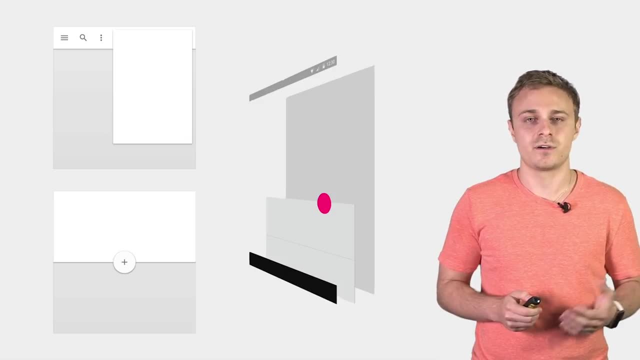 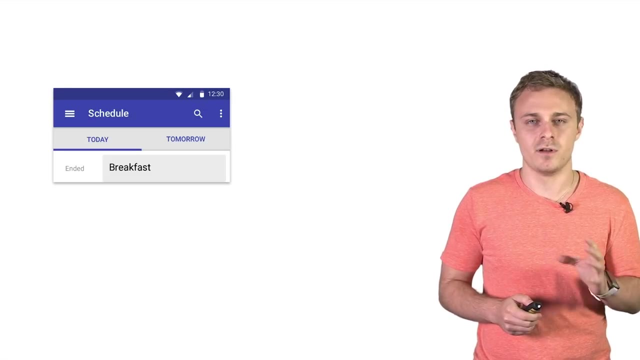 decisions like where shadows should appear and what is drawn on each surface, For example. here's our first iteration of tabs in the My Schedule screen. It was problematic for a number of reasons. The single shadow below the action bar conveys that there are 2 sheets of paper, one for. 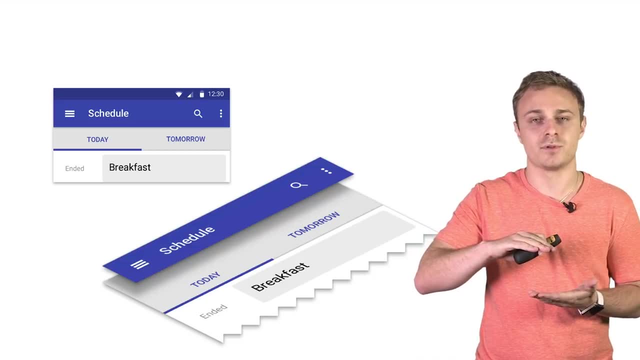 the action bar and one for the tabs and schedule content. The problem is that the bottom sheet is too complex. The ink that represents the contents of a surface should be pretty simple. Here ink is doing too much work, painting not only text and icons but borders and background. 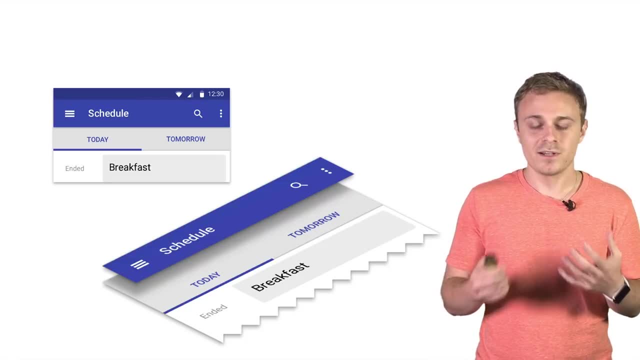 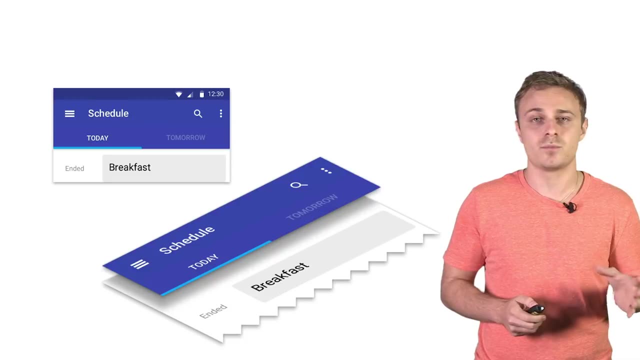 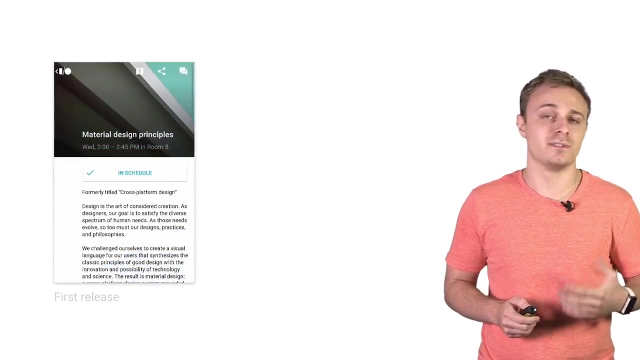 colors. The result is visual noise. Our final iteration was much stronger, creating a clear separation between colors and the lower part of the screen, But the pattern really did between chrome and content and letting the ink focus on painting only the important stuff, things like text, icons and accent strips. another area where surfaces played a role in our design. 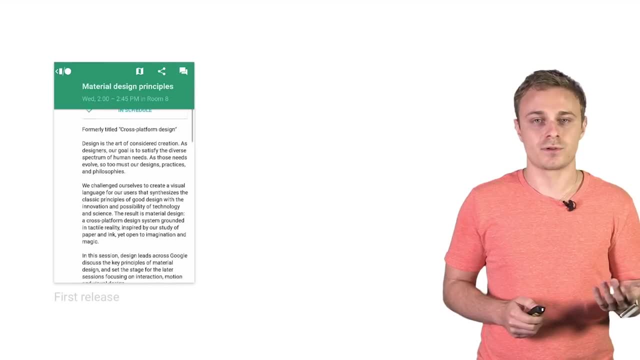 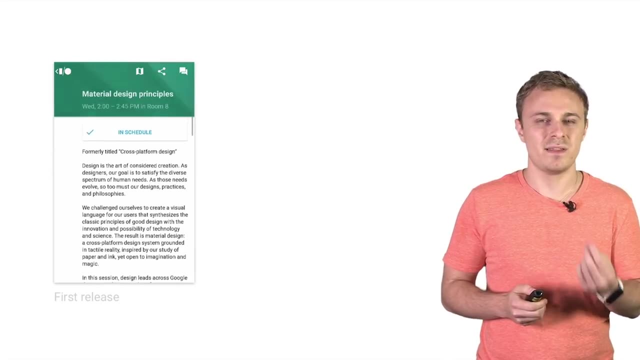 thinking was a detail screen in our first release. as you scroll, the top banner cross faded between the session image and the session color. our concern, though, was that this design bent the physics of material design too far. it's as if the text was sliding along a surface whose transparency 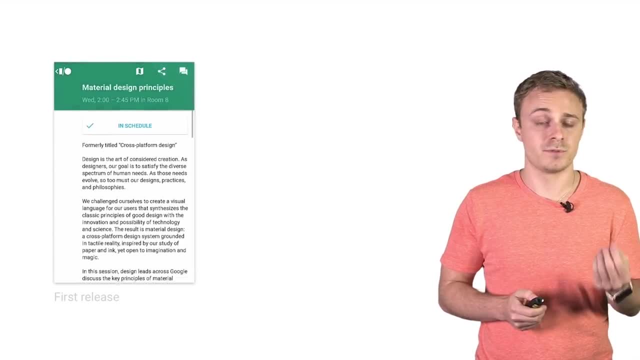 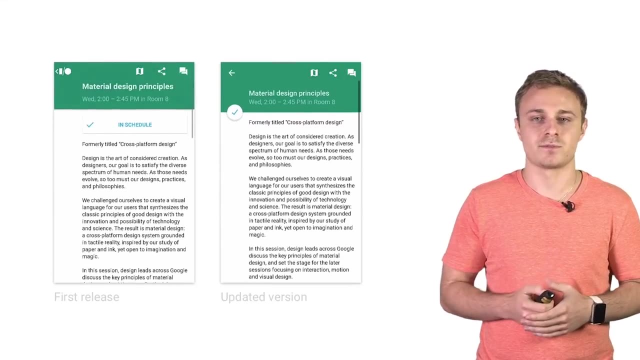 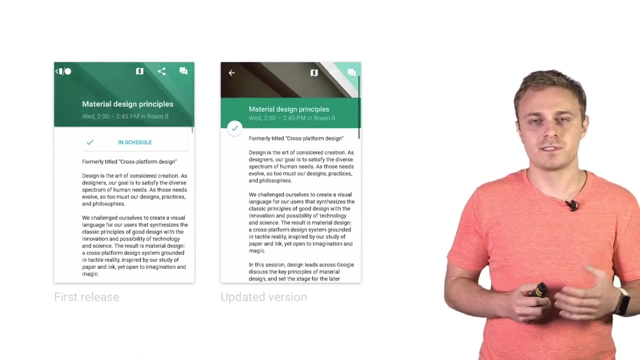 changed throughout the animation. a better approach, which we introduced in an update to the app on june 25th, was to create a shorter surface below the image onto which the title text was printed. this surface had a more stable opacity before scrolling. the surface is adjacent. 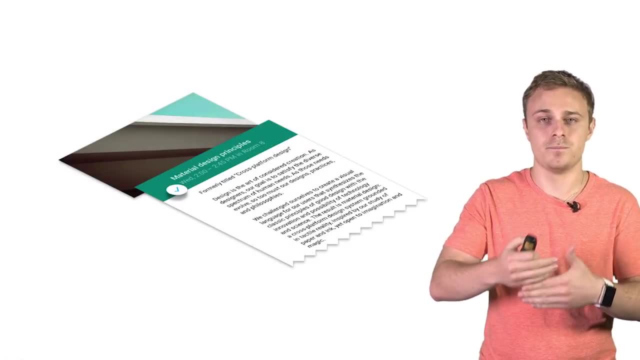 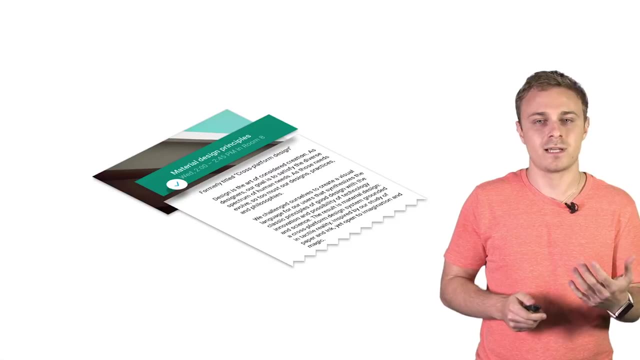 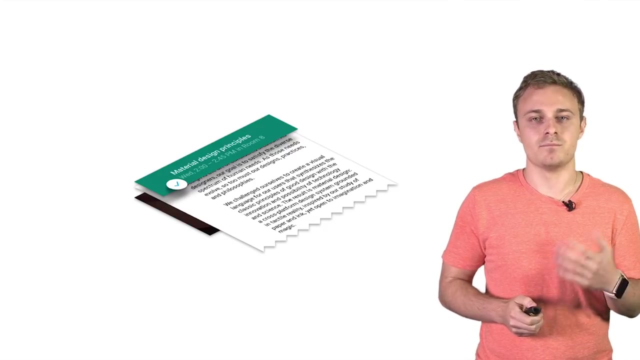 to the one containing the body text, forming what we call a seam, and as you scroll, this surface and the floating action button attached to it rises above the body text, allowing the text to scroll beneath it. this aligns better with the physics in the world of material design and the end result is a more 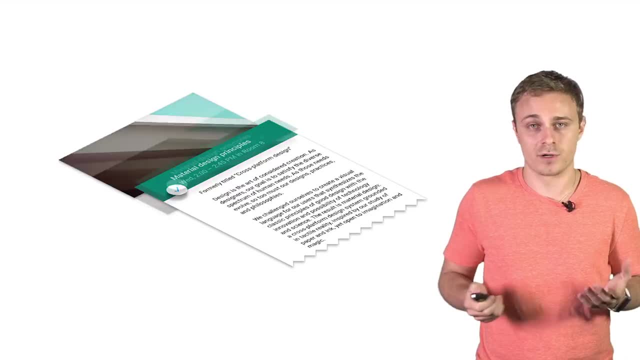 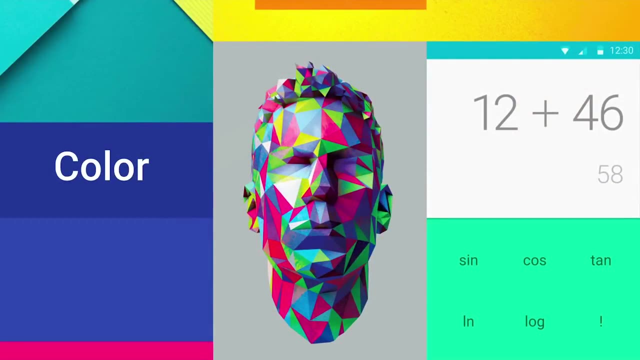 coherent visual interaction and motion story for our users. now, another key principle of material design is that interfaces should be bold, graphic and intentional, and that the foundational elements of print design should guide visual treatments. color plays a huge role in making that happen. in material design ui color palettes generally consist of one primary 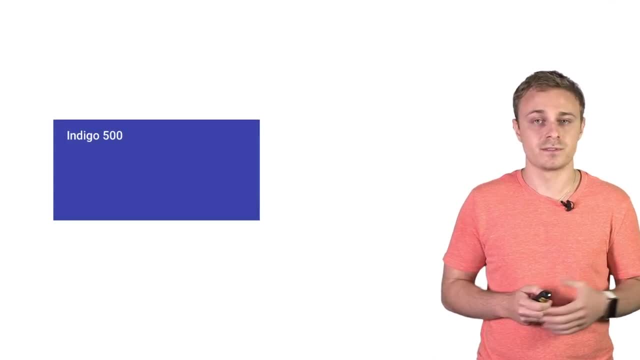 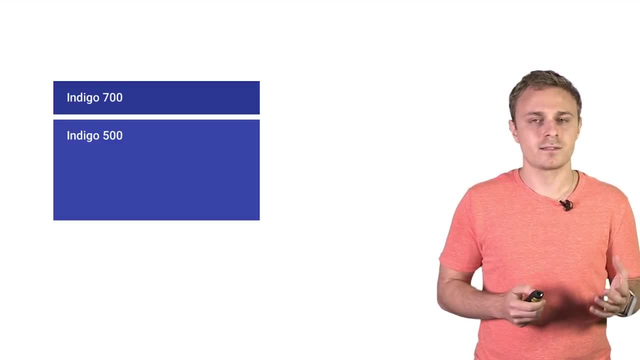 shade like the 700 value. the accent color is used more subtly throughout the app to call attention to key elements. the resulting juxtaposition of a tamer primary color and a brighter accent color gives the app a bold, colorful look without overwhelming the app's actual content. 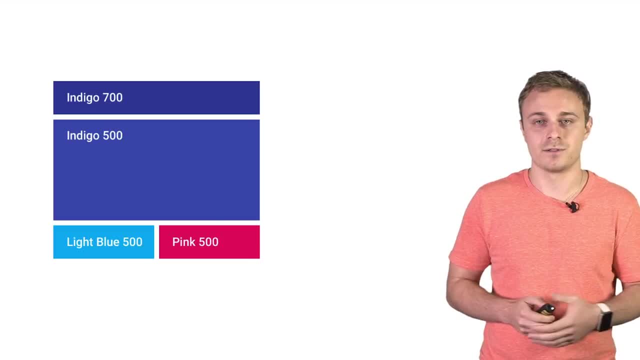 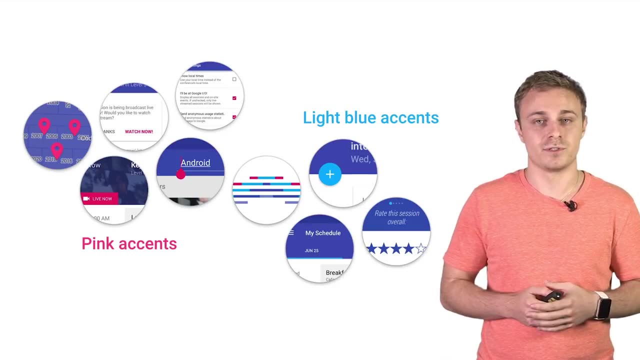 in the i o app, we actually chose to use two accent colors used in various situations. most accents were pink 500, while the more conservative light blue 500 was a better fit for the add to schedule button, which was often adjacent to session colors. and speaking of session colors, 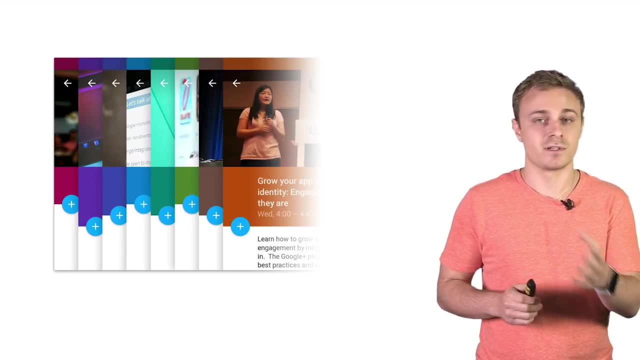 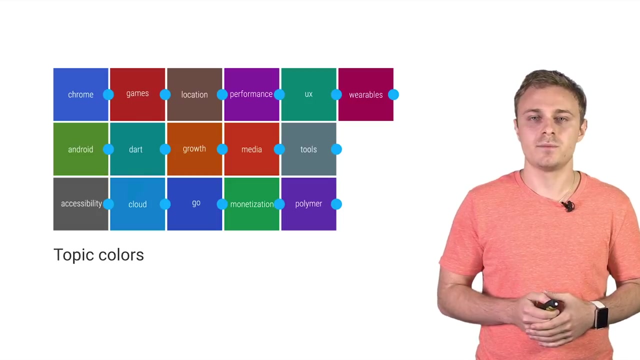 we color the detail screen based on the session topic. for example, android sessions are green. this gives the screen that bold and intentional look, and when choosing our topic colors, we use the material design color palette, which contained dozens of great color options. we also needed to make sure that each color contrasted well enough with the floating action button and session images. 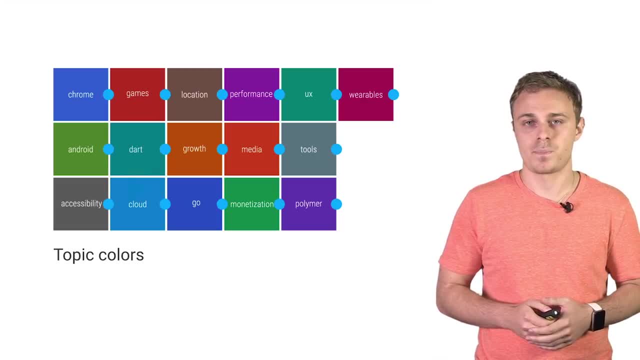 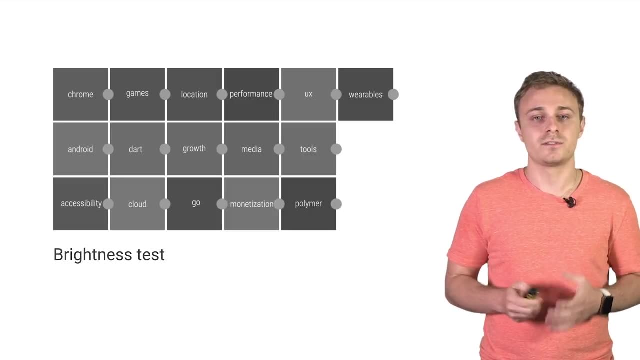 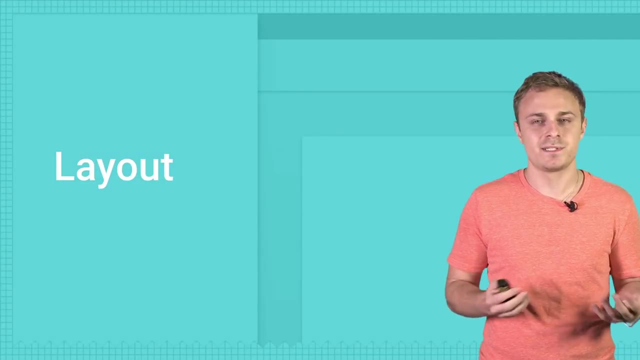 here's our test graphic that let us visualize this contrast. finally, we ensured that topic colors had a consistent brightness. desaturating our test file when choosing the colors helped in that process. now, another foundational element of print design that's important in successful material design is layout and, more specifically, margins and what we call key lines. now from previous years of the 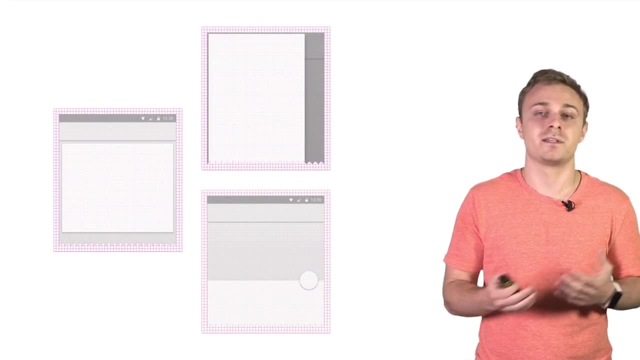 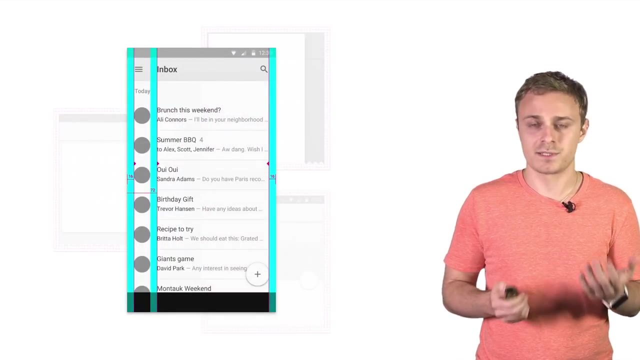 i o app. we'd already been accustomed to using a four dip grid for sizing things. for example, our buttons and list items were 48 dips tall. however, the guidance on key lines from material design was new to us after we started adhering to the spec and, in particular, aligning titles and other. 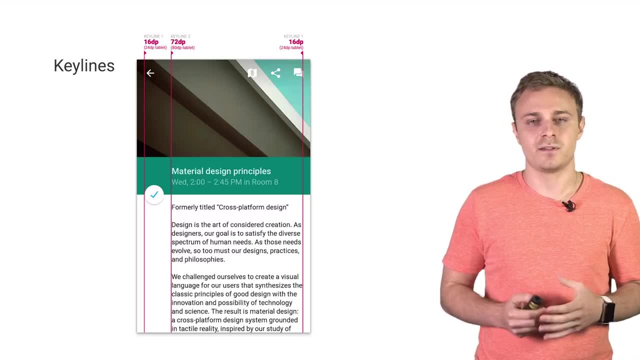 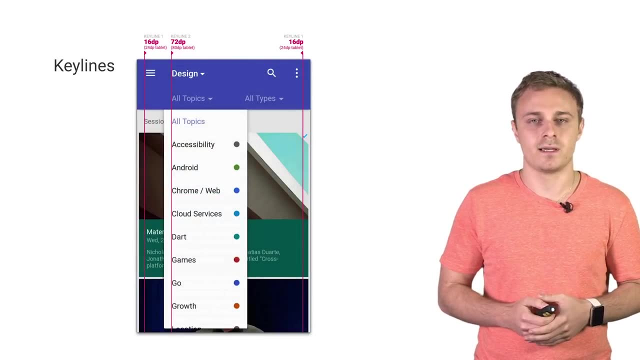 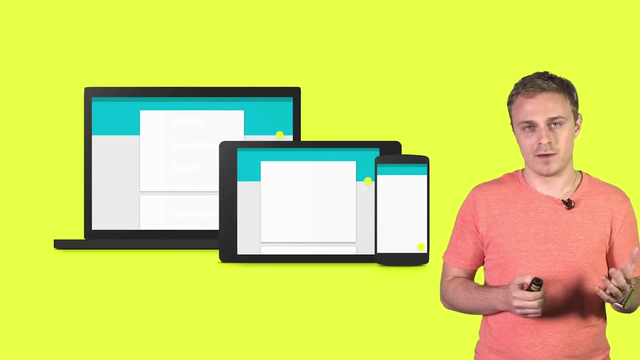 text to that 72-dip key line. we immediately felt that clean, print-like rhythm in our screens. adhering to the key line allowed for very fast scanning of ui text and information on our screens. gestalt principles for the win. now, while we're on the subject of layout, remember that 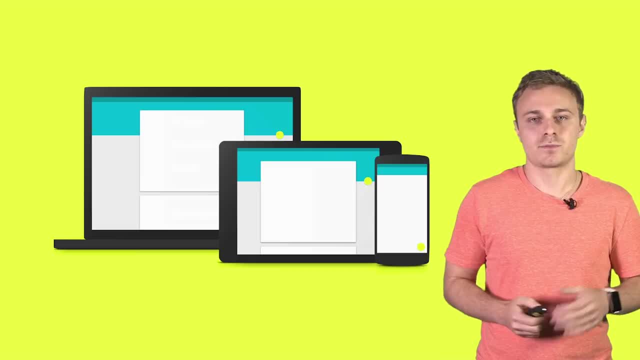 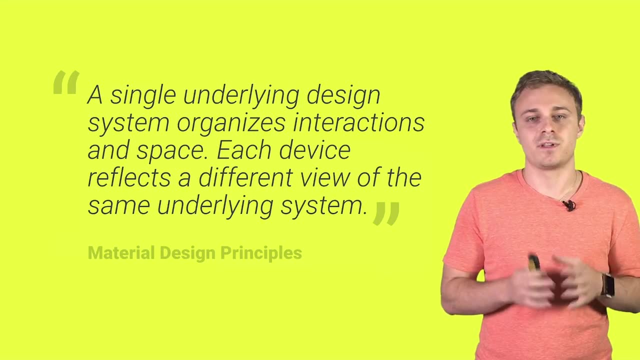 material design applies across many device types. it's right there in the principles. a single underlying design system organizes interactions in space. each device reflects a different view of the same underlying system. now, luckily, the spec offers some great solutions for designing across different screen sizes. for example, many of the screens in the i o app represent collections of 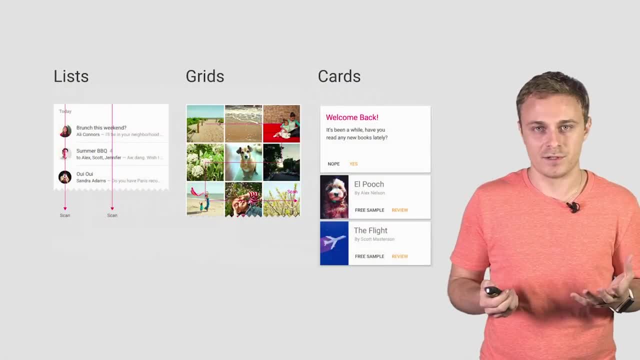 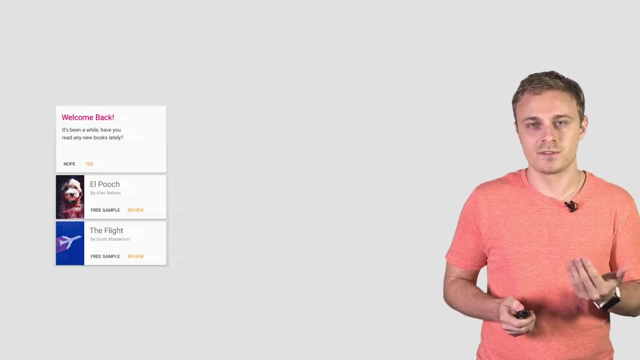 sessions. for these situations, the system offers a number of containers like lists, grids and cards. each of these can be used across different screen sizes to represent collections of data. we originally thought to use cards to represent session items. it's a pretty natural choice, but in some cases we wanted to conserve space by overlying overlaying text and images. this simpler. 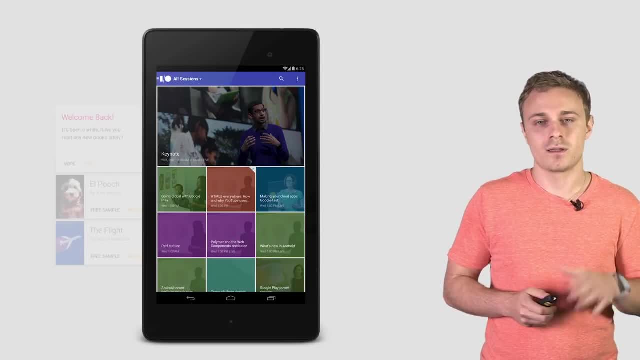 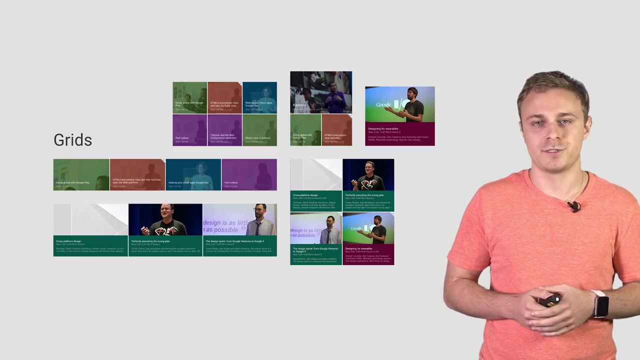 more homogeneous presentation cards. the card shadows and corners would hinder the scannability. in this context, we thought a grid would be a better choice here. with grids we could vary the number of columns based on available screen width, and each grid tile could take on different aspect ratios. the 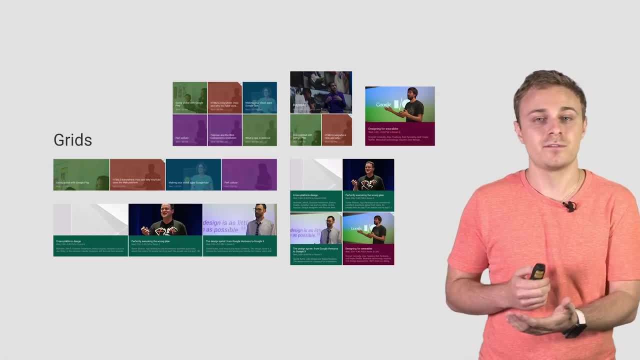 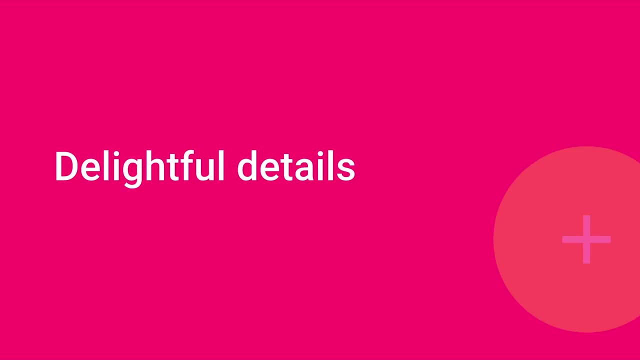 resulting presentation was very flexible and worked great, not only on phones, but also 7-inch and 10-inch tablets. finally, there's a crucial element that ties everything together, and that's motion. while a big part of the motion story is that it's not just about the screen size, it's also about the 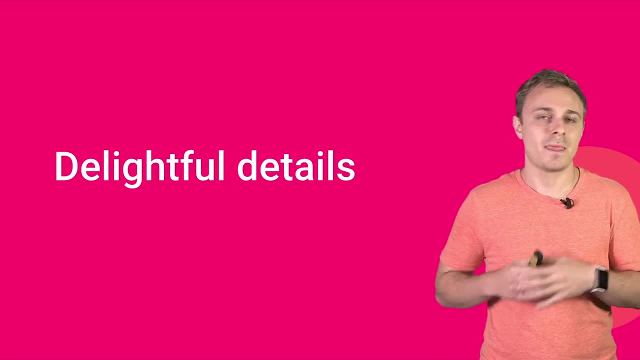 application size. so even though the motion story of material design is in transitions between screens, apps can truly delight users when motion is used in ways beyond the obvious. let's take a look at some of the delightful motion we introduced in the app. first touch feedback: ripples they're.